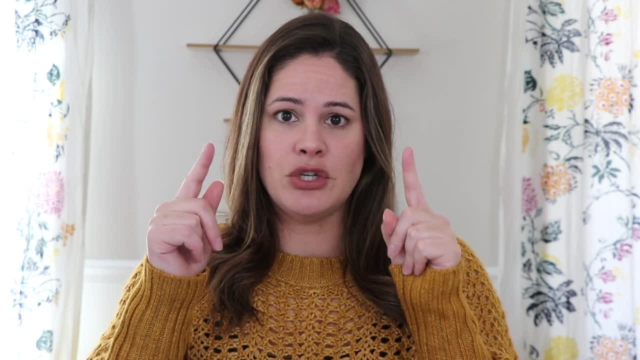 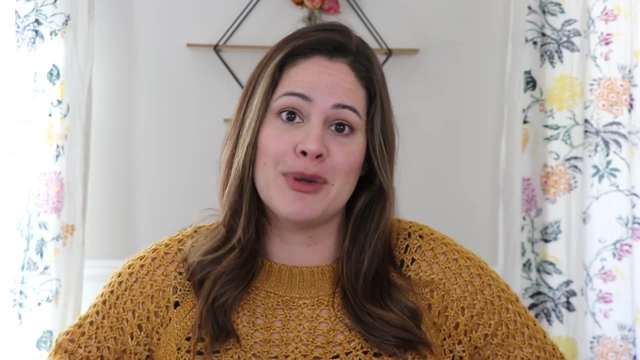 about that. The page will actually have links to both my writing club and my math club, so you'll see when you go on there. when it's a picture of writing and a picture of math, just click on the math one if that is what you want to learn more about, As I've been creating these math activities. 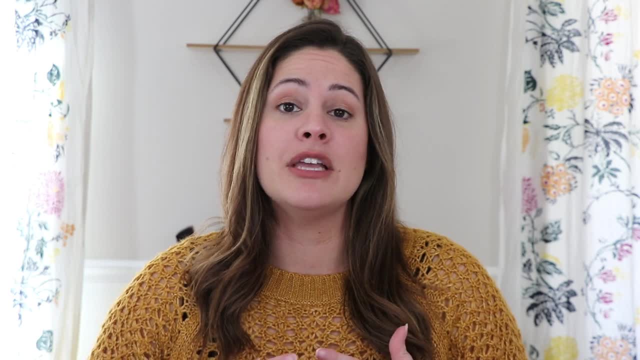 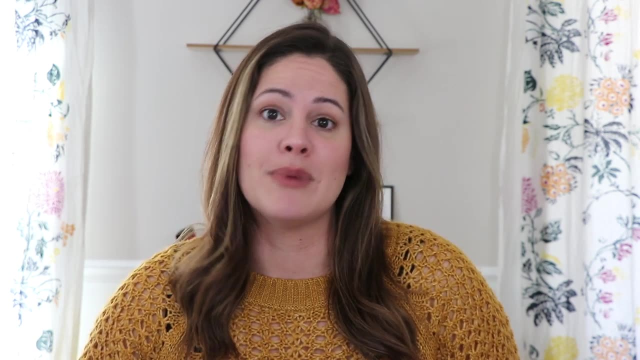 and getting excited for it. I thought to myself I haven't shared these two, like I said, really easy and fun hands-on addition activities that I actually recently just completed with both of my friends at home. I should also mention that both of these hands-on addition activities are great for. 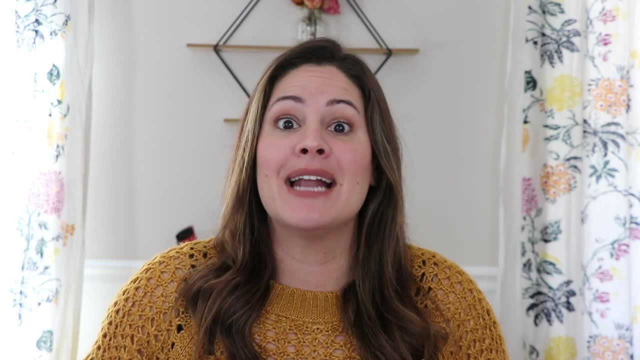 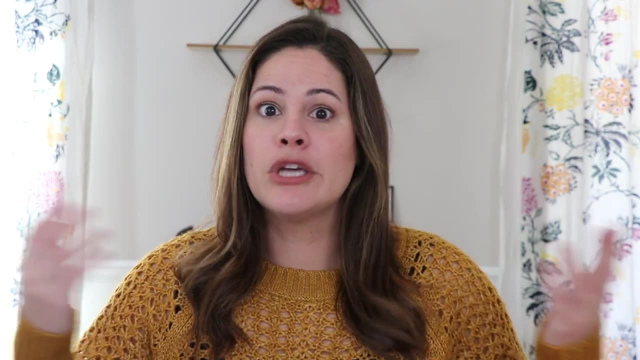 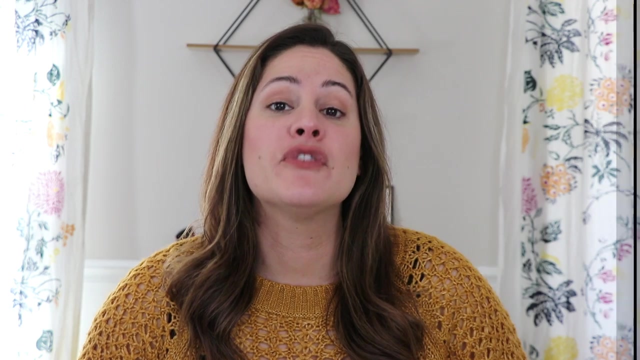 students that are either heading into kindergarten or maybe had kindergarten this past year, and they're fun ones to just send along to your parents so they can do them over the summer. So, without further ado, let's see how to play. The first one I want to share are just these build-it cards. Now, I'm sorry if there's a glare. 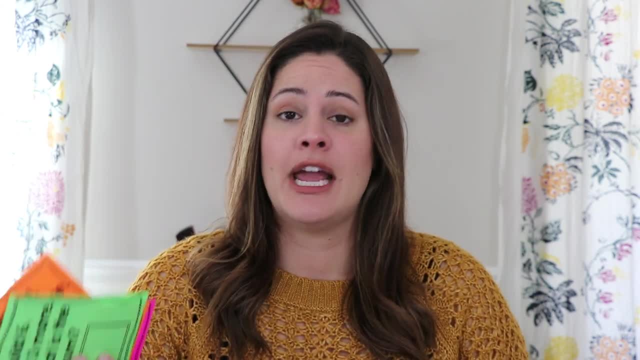 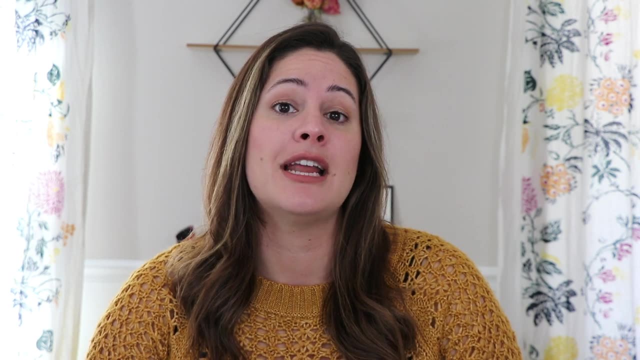 because I have mine laminated. but these build-it cards I actually had for free on my blog for like seven, eight years now, and they're something that I created for my kindergarten and first grade students, I think back in 2012 or 2013.. So it is a. 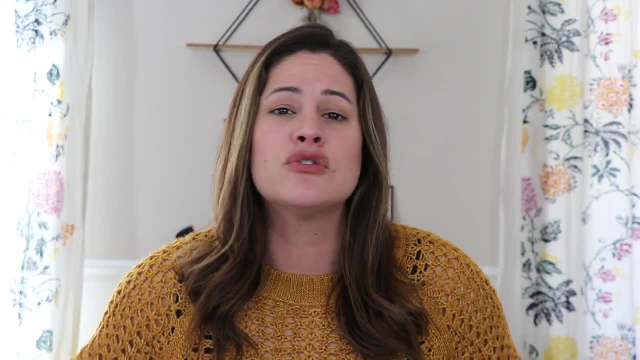 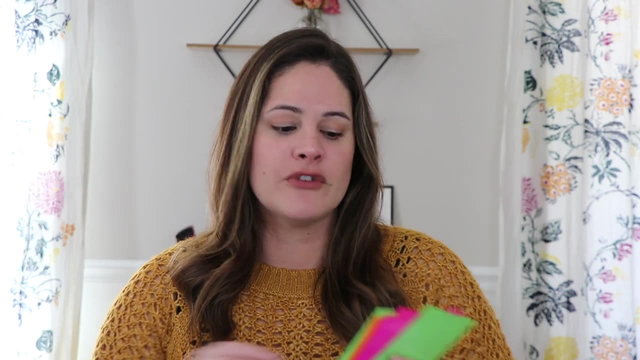 very simple activity where students- this is kind of when they're just getting introduced to addition or if they need some remedial practice on addition. When I was making these cards I just thought it was an easy way for students to visualize addition and adding one part and another part together to 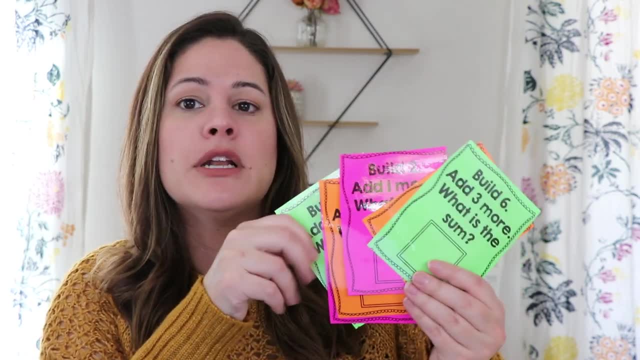 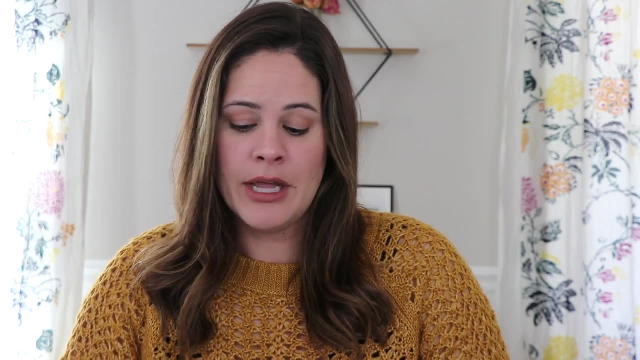 create a sum. So basically I eliminated these cards on some, you know, colorful paper to make them more fun and interesting, but all students will do. there's a bunch of different cards. I think there's 20 of them, So students would just pick a card. 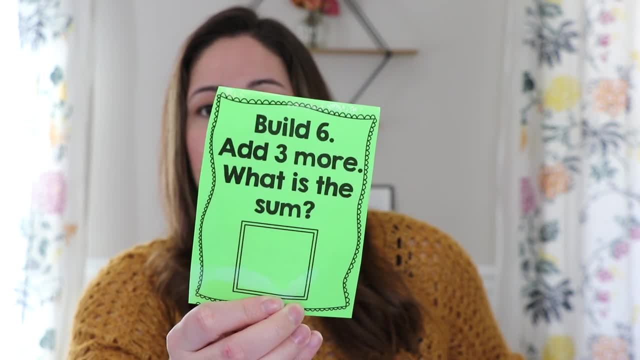 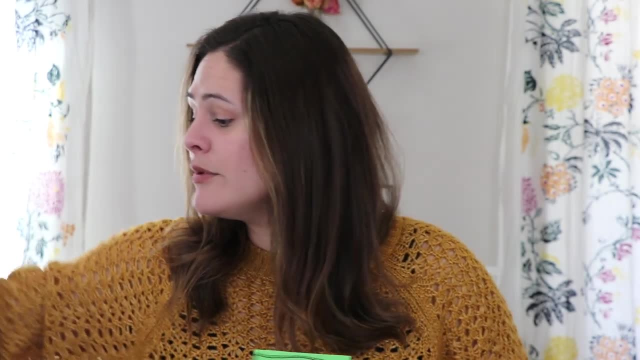 Let me see if I can get it in there so you can focus on it. There you go. So the first part says build six. So all they would need to do is go ahead and grab. in my class we would use connecting cubes like these. I have a whole pile over here. 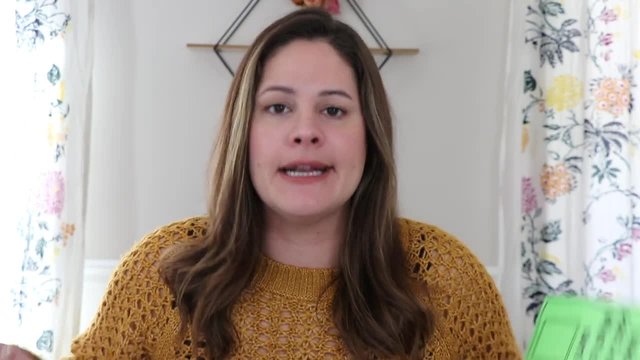 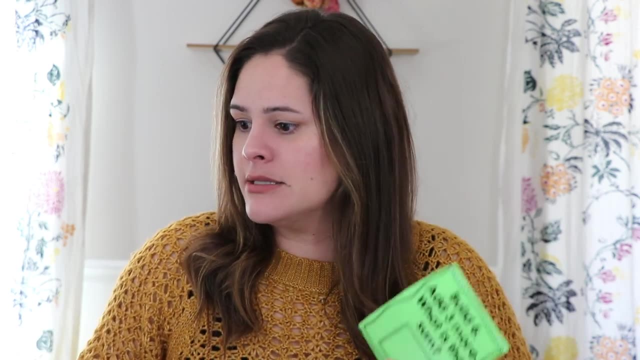 But if you don't have these at home, you could easily just grab anything. So six of eight, They can either build it or they can collect it. So it could be Cheez-Its, goldfish buttons, any small little manipulative that you have at home. 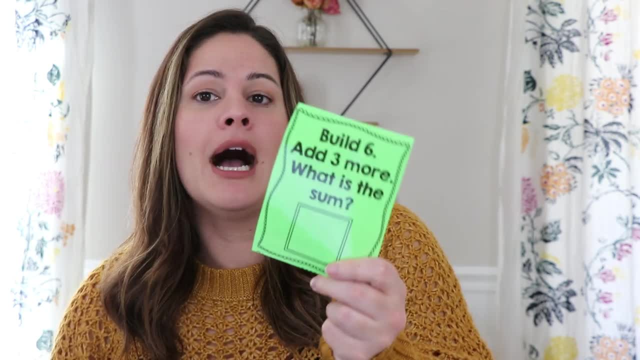 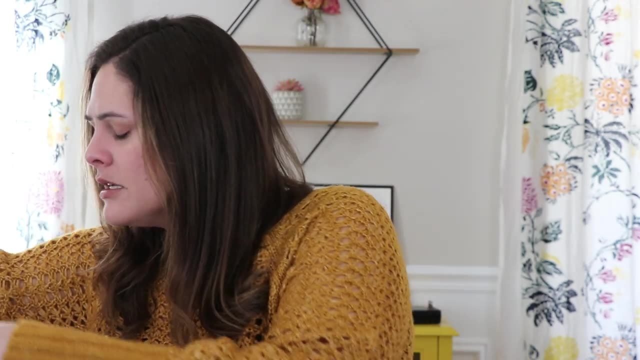 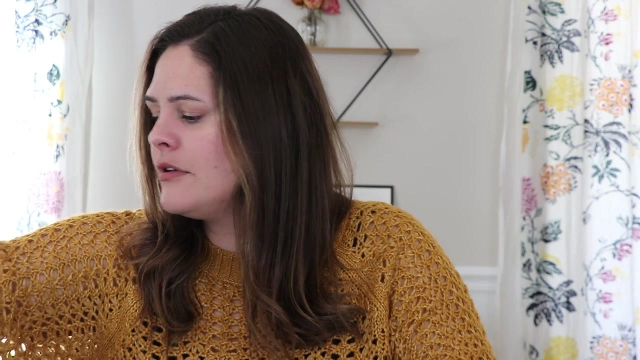 So in the classroom though- and you might want to carry this over at home- I would have students build six with the same color, So they would go ahead, and that was their first step: Build six. So I'm going to grab six red One, two, three, four, five, six. 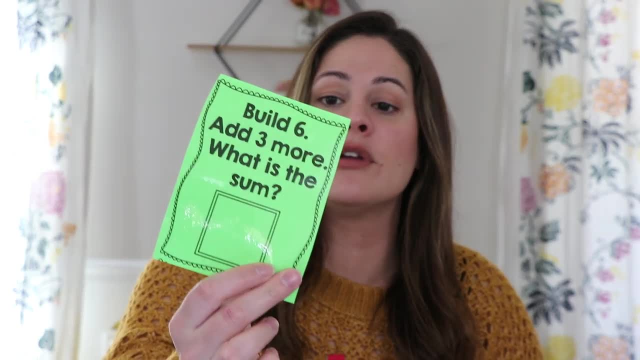 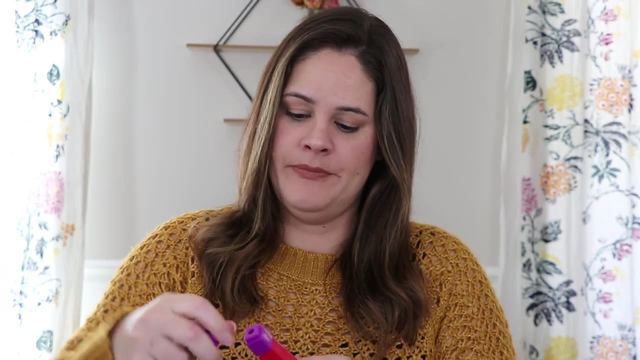 Build six. Next it says: add three more. What is the sum? So they would grab a different color. Let's grab purple One, two and three to make their little tower, And then I would say what is the sum. 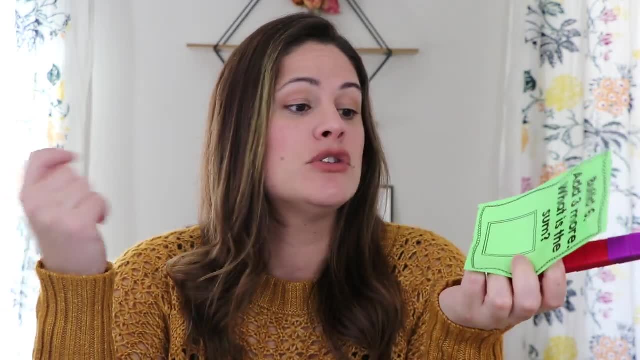 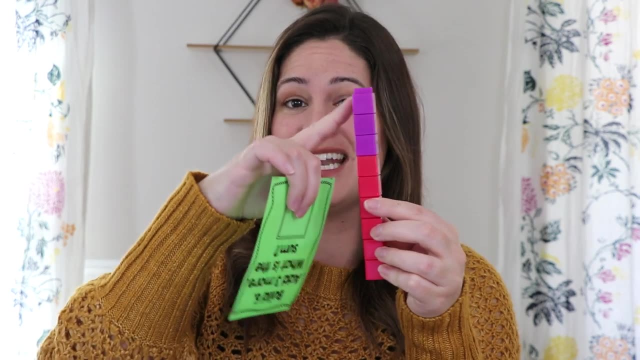 And the reason I went ahead and laminated these is because I would always have my students do it with a dry erase marker, So they could actually just go ahead and write all right: one, two, three, four, five, six, seven, eight, nine. six plus three equals six. 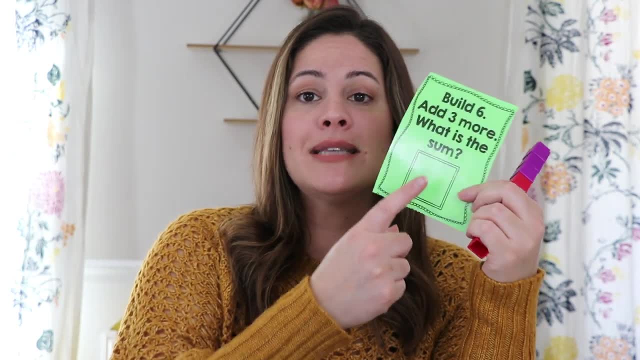 One, two, three, four, five, six, seven, eight nine. six plus three equals six. One, two, three, four, five, six, seven, eight nine. six plus three equals six nine. So they would write the sum right here, They would put their card down and I would when 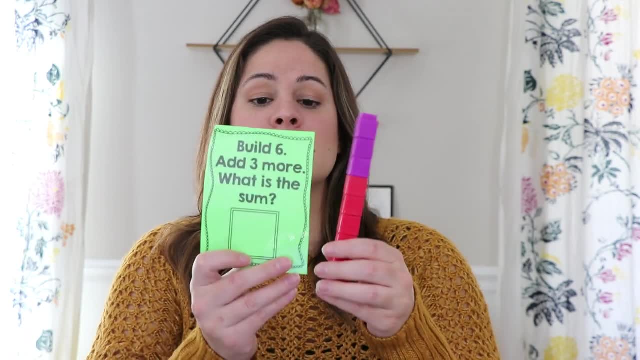 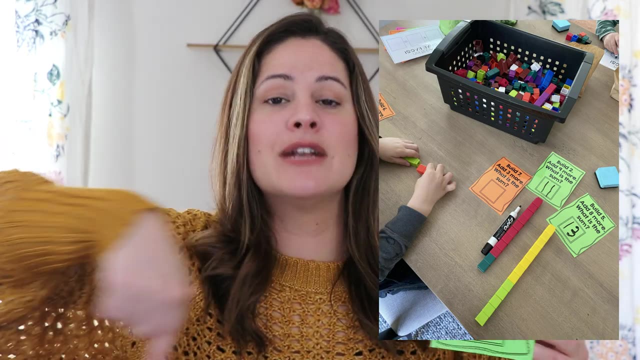 they're doing this like independently at centers. I would always have students leave their card next to the cubes for just a little bit. They always had to leave at least like three out at a time. so when I was kind of walking around I could quickly just double check on the students. 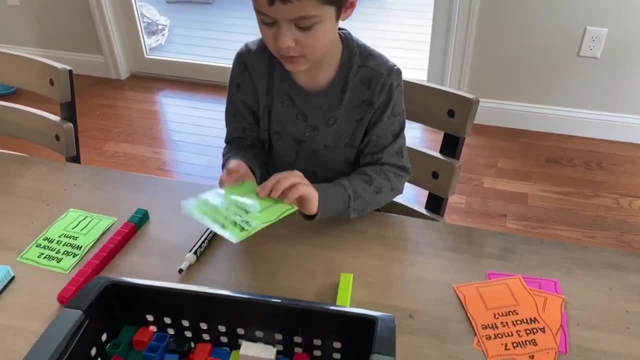 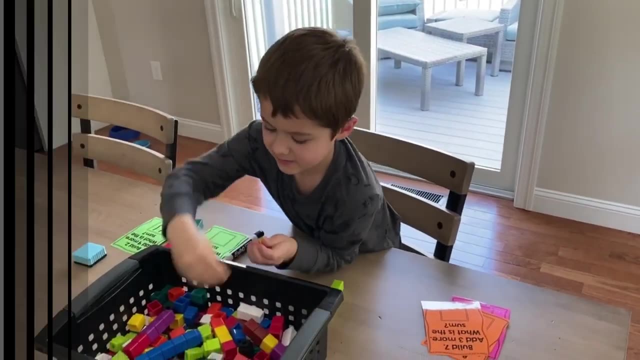 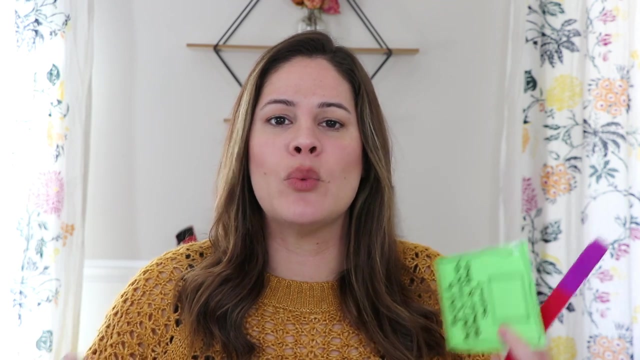 answers: Add eight more. I have to add eight. I'm gonna do eight yellow. Another reason I loved using these at the beginning of the year in the classroom was it was a great way for me to kind of walk around and assess where students are at in their edition, You know, are they still using? 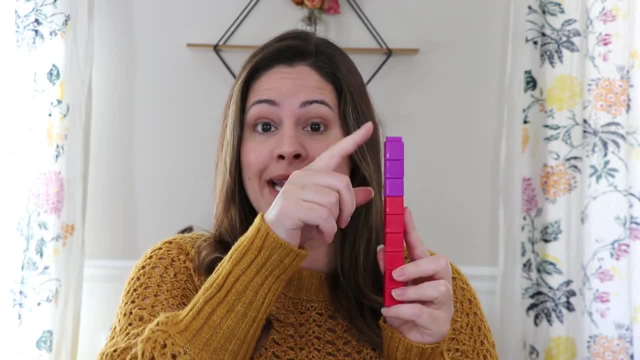 one-to-one correspondence. when they're counting up those six cubes and then adding three more, When they're finding the sum, are they able to just quickly add on? Are they able to just quickly add in more? Are they able to just quickly add in more? Are they able to? 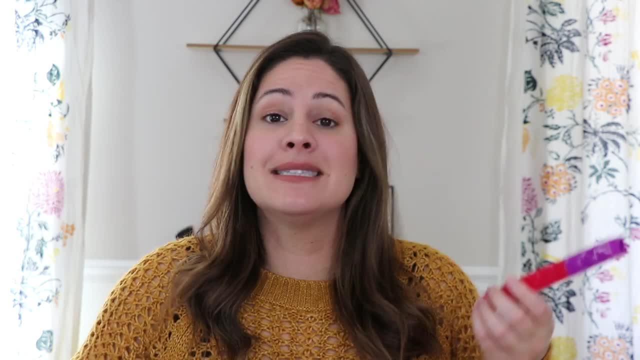 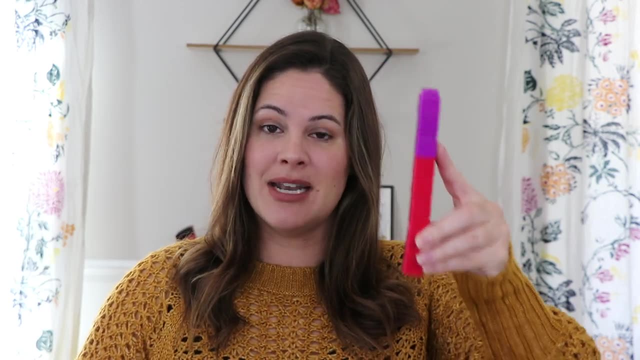 to say, okay, I know there's six here, so seven, eight, nine, and some of them will already know they'll say, oh, build six, three more, I know that's nine. they'll still do it and actually build it and show it so they can see what nine and the six and the three part looks like. but you'll just be able. 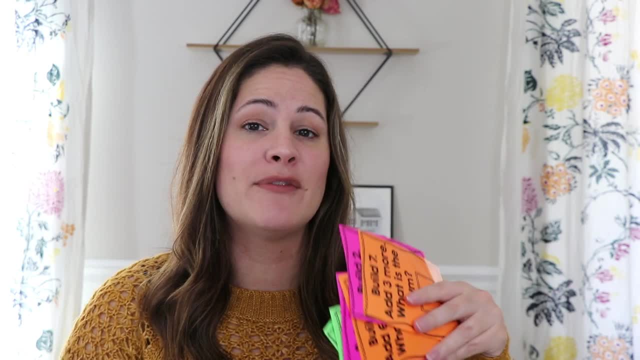 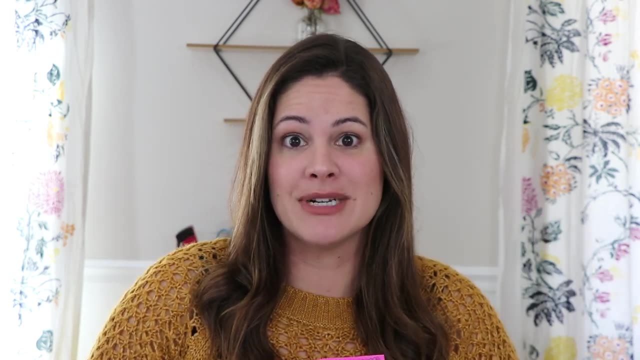 to quickly assess kind of where your students are at. like I said earlier, I have about 20 of these cards. I will link them down below with the other game, so after this video you can go ahead and grab those and print them out. all right on to addition activity number two. this is another hands-on one. 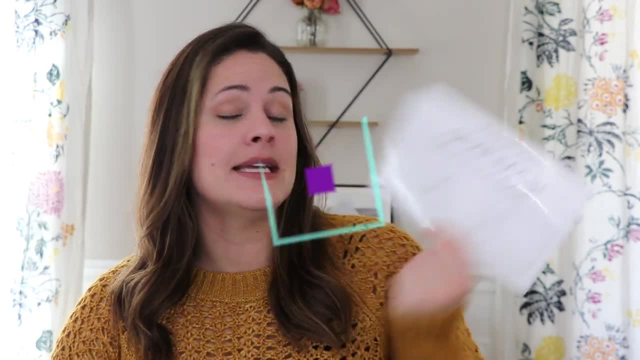 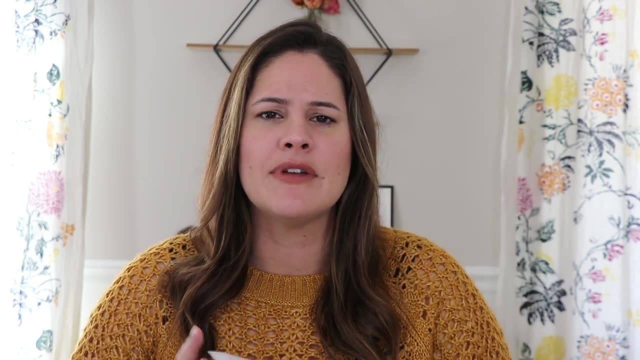 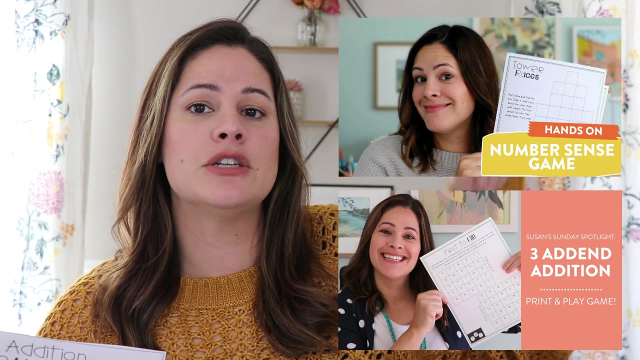 called addition grab bags, and this is a very simple activity. I've actually included it. it's in a packet that has like 19 pages and, I think, seven different activities. so I've talked about this unit a couple times. it's again a free unit that I have and I'll go ahead and show some of the 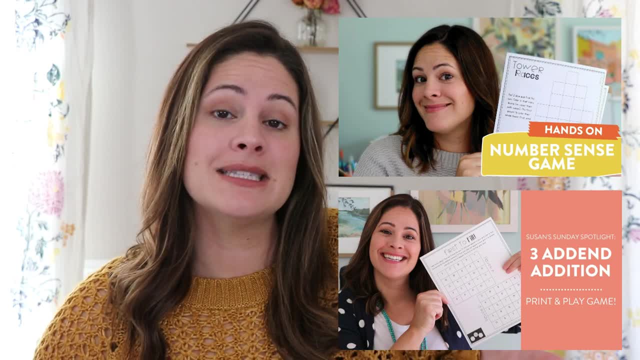 thumbnails of other videos where I talked about different activities in this. so if you've actually downloaded this card, you'll see that it's a very simple activity and I've included it in a packet. you may have already seen this activity, but in case you haven't, I wanted to share it. 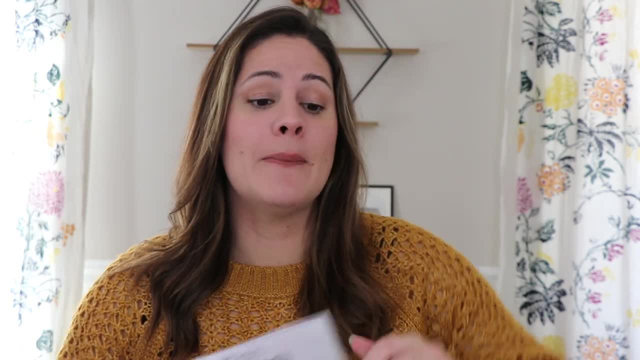 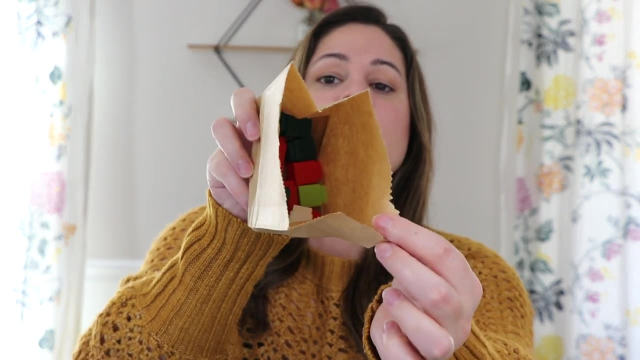 today. addition, grab bags is as easy as it sounds and basically you're going to have two bags filled with some sort of manipulative. so in here- I don't know if you can even see this, but in here I have some cubes- the same type of cubes I had for the last one- and I like this because you can easily 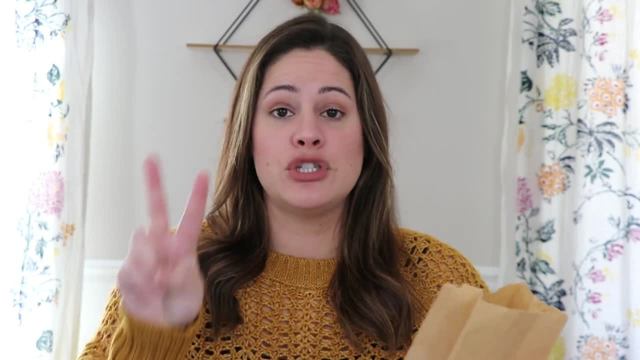 differentiate it for whoever you're playing with. so you're going to have two bags, so you'll have to decide what addition you want to practice within, whether it's addition within 20, addition within 20 or whatever you want to practice within, whether it's addition within 20 or whatever you. 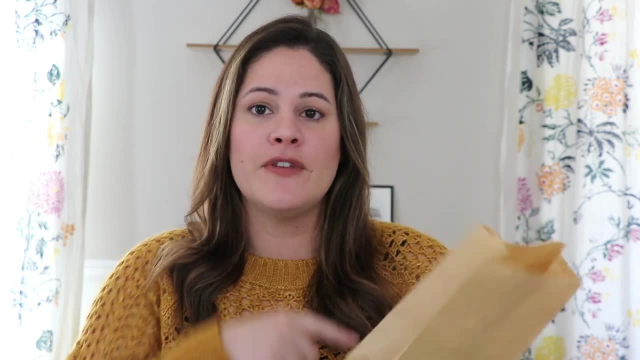 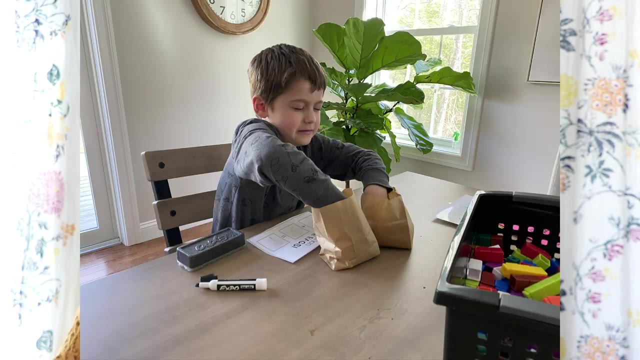 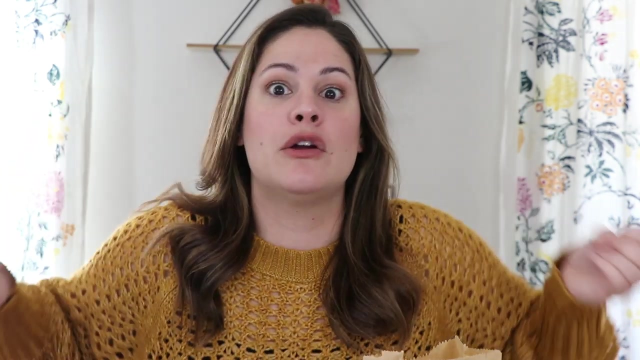 want to practice within 10. it's up to you, so you'll decide. I have about 15 cubes in this bag and 15 cubes in the other bag, and all students are going to do is they will take a minute, they will close their eyes, put them in each of the bags and they'll grab some cubes. so addition: 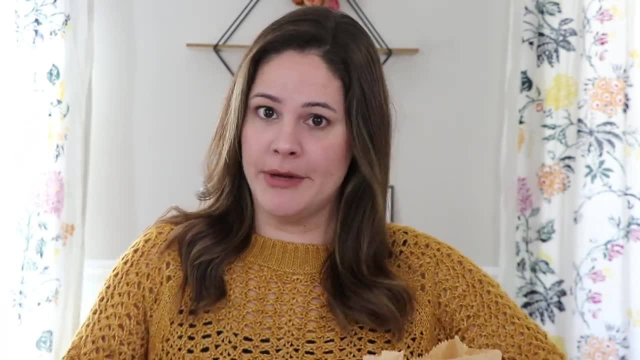 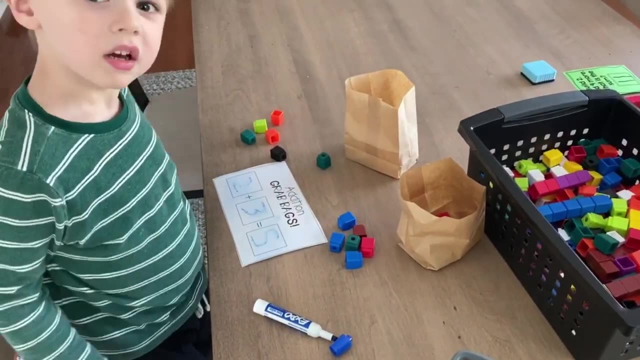 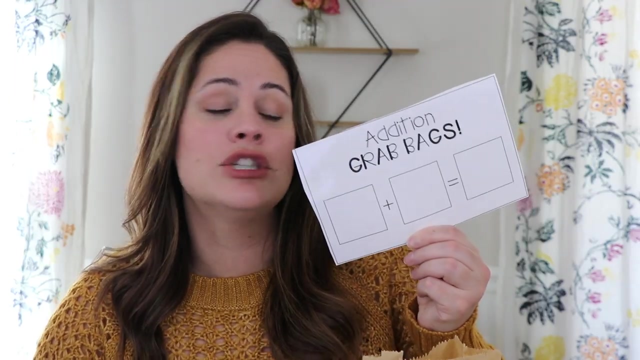 grab bags. they'll basically grab some cubes in each of their hands, put them on the table and then find their sum. oh goodness see how many: one, two, three, four. here's the recording sheet that they can go ahead and use again. I laminated it so they can use a dry erase marker. so if they grabbed six from one, 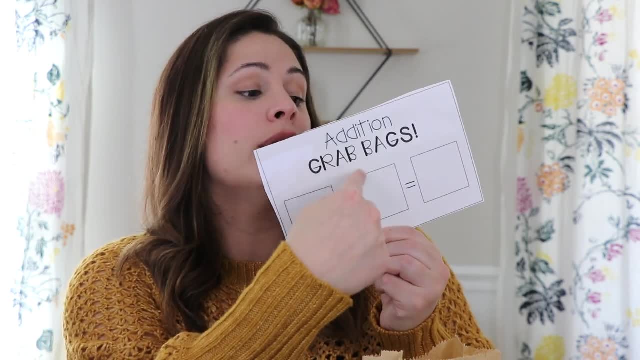 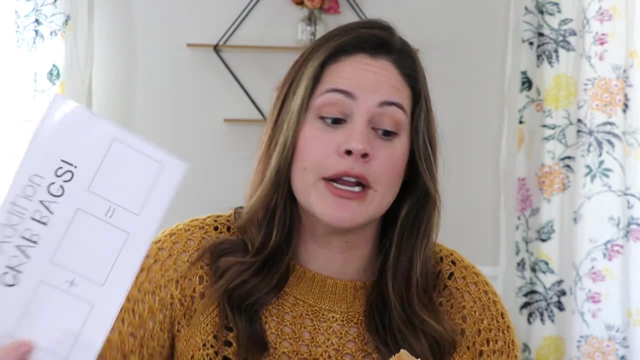 bag and seven from another. they would write six plus seven. they would count up the sum and write it right there as 13.. now I do have these that are laminated in case you wanted them to practice it over and over, but also if you were in the classroom or even if you just wanted to practice a bunch of